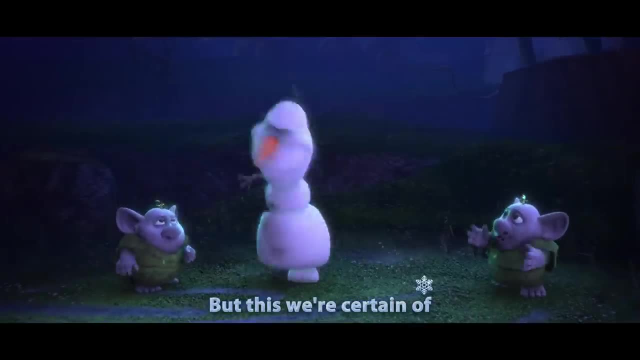 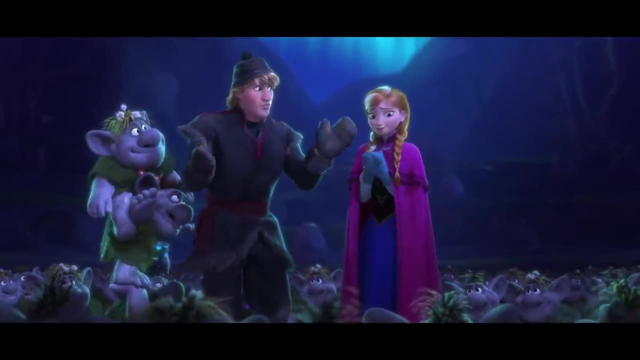 So he's a bit of a fixer-upper, but this we're certain of, You can fix this fixer-upper up with a little bit of love. Can we please just stop talking about this. We've got a real, actual problem here. 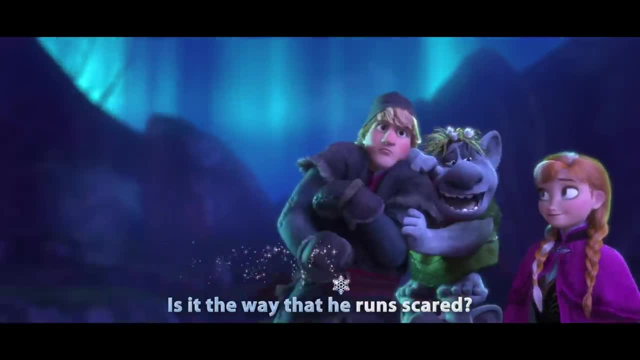 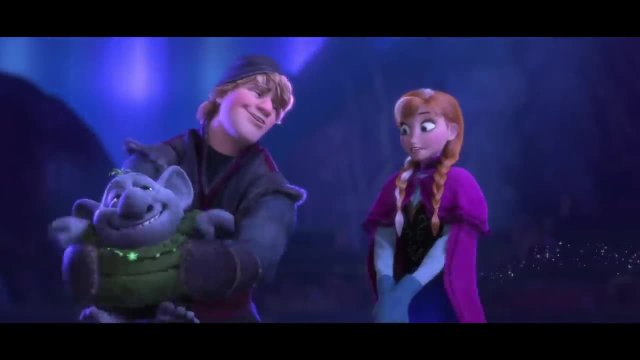 I'll say: So tell me, dear, is it the way that he runs scared, Or that he's socially impaired, Or that he only likes to tinkle in the woods? What, What Are you holding back your fondness due to his unmatchly blondness? 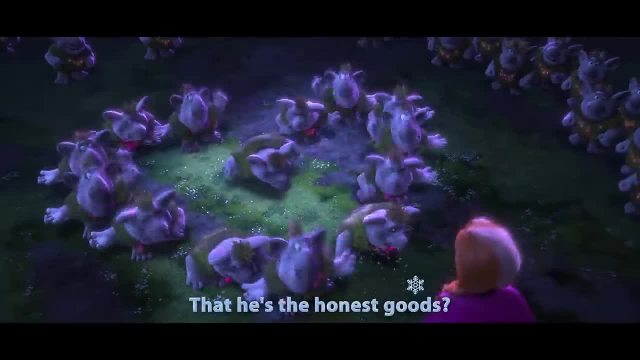 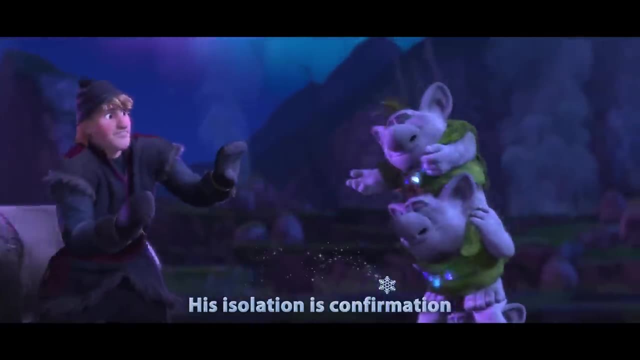 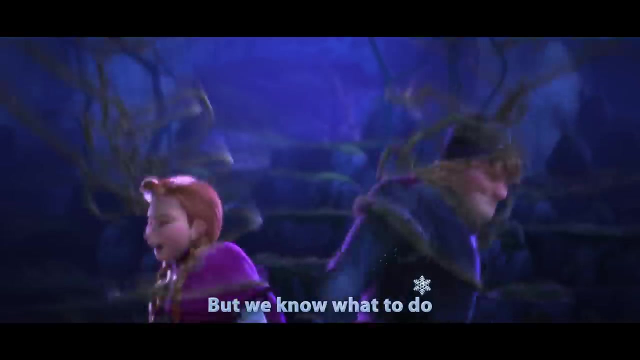 Or the way he covers up. maybe he's the honest goose. He's just a bit of a fixer-upper. He's got a couple of bugs. His isolation is confirmation of his desperation for a healing hut. So he's a bit of a fixer-upper, but we know what to do. 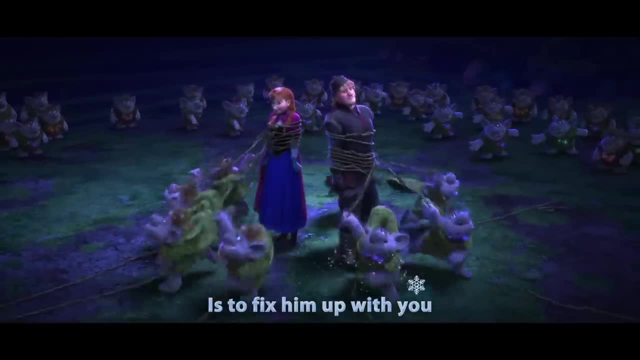 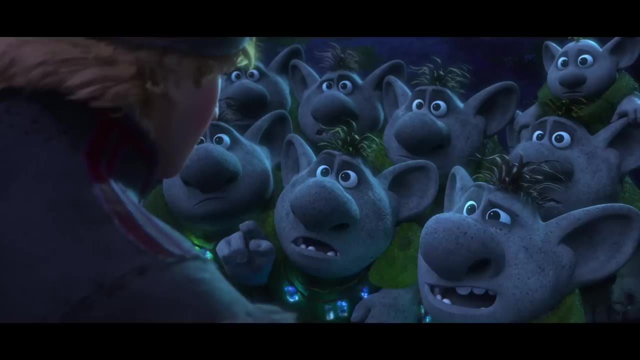 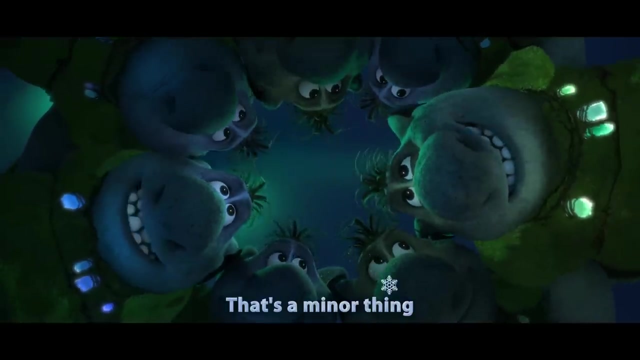 The way to fix up this fixer-upper is to fix him up with you Enough. She is engaged to someone else okay, So she's a bit of a fixer-upper. That's a minor thing. Her quote: engagement is a flex arrangement. 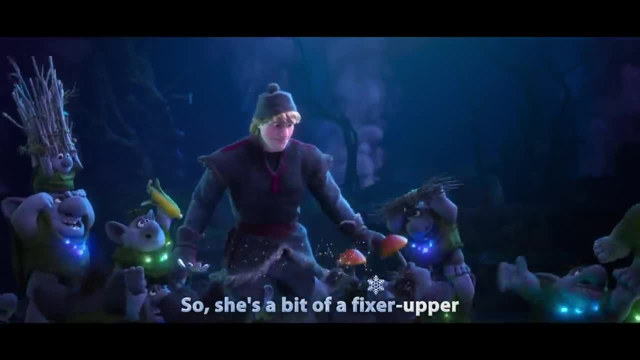 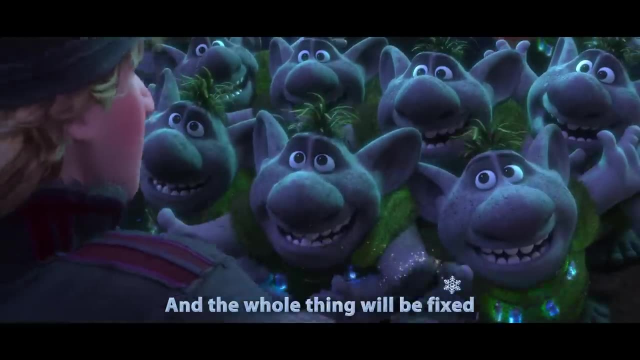 And, by the way, I don't see no ring. So she's a bit of a fixer-upper. Her brains have been betwixt. Get the fiancé out of the way and the whole thing will be fixed. We're not saying you can change him. 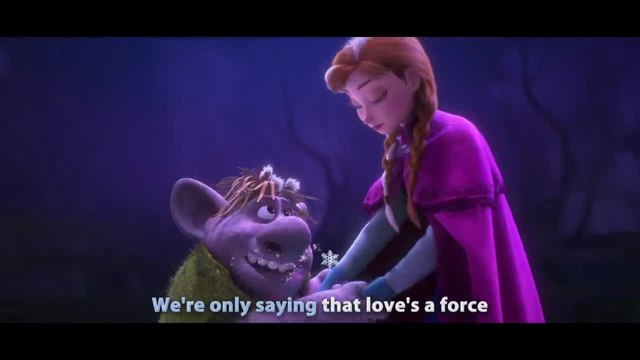 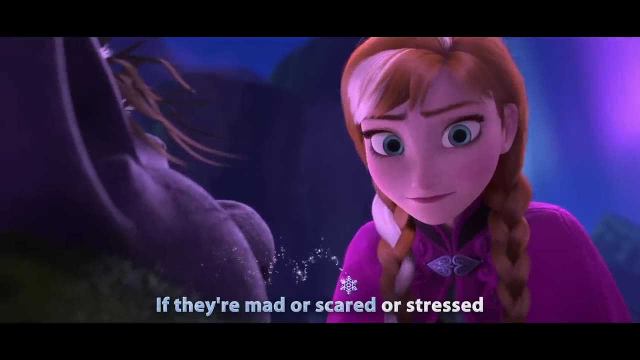 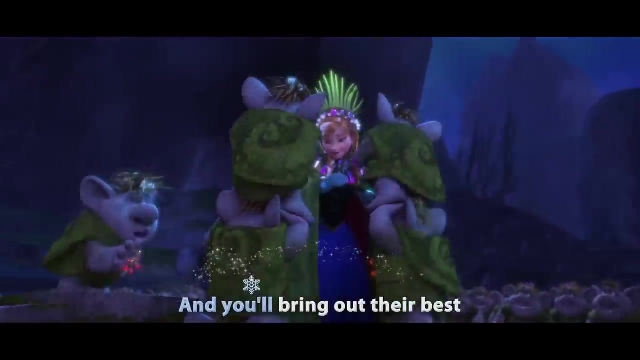 Because people don't really change. They're only saying that love's a force that's powerful and strange. People make bad choices if they're mad or scared or stressed. Throw a little love their way. You'll bring out their best. True love brings out the best. 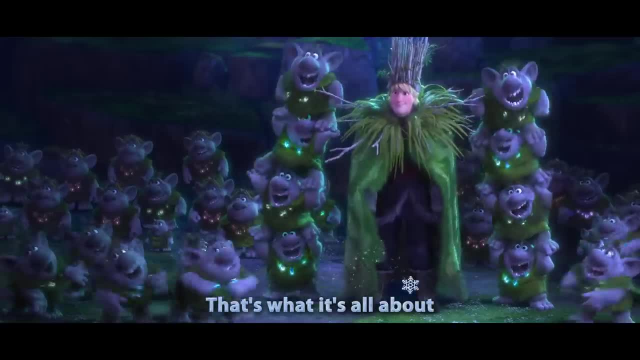 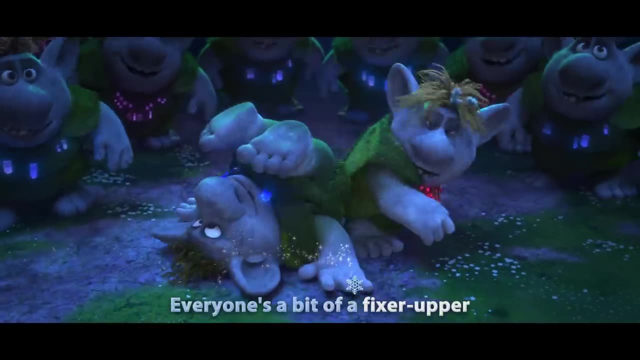 Everyone's a bit of a fixer-upper. That's what it's all about. Father, Sister, Brother, We need each other to raise us up and round us out. Everyone's a bit of a fixer-upper, But brainwash gots to show. 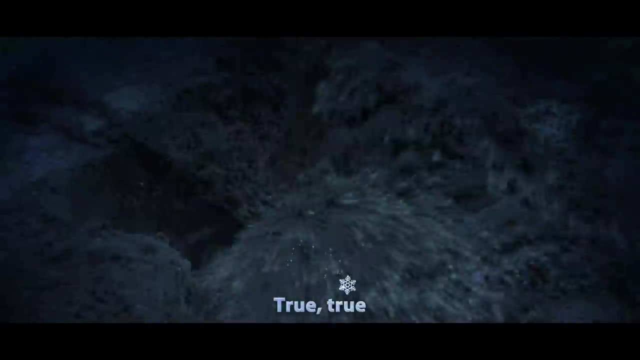 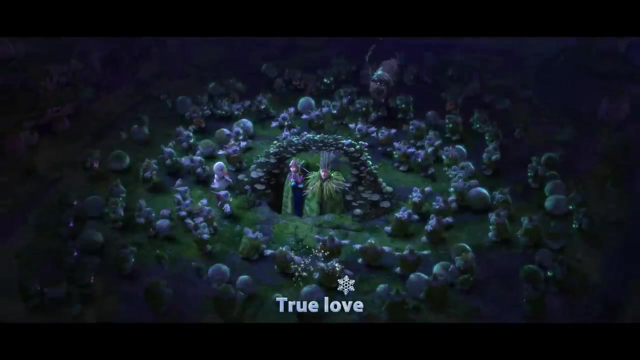